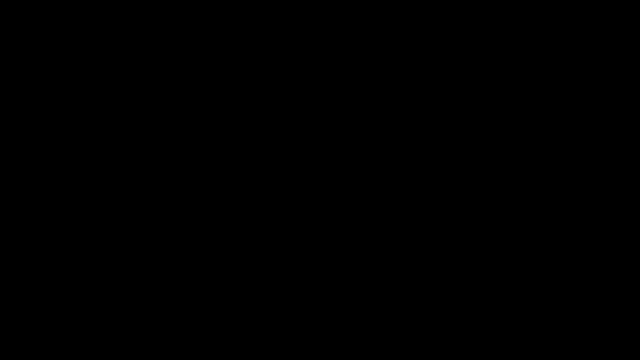 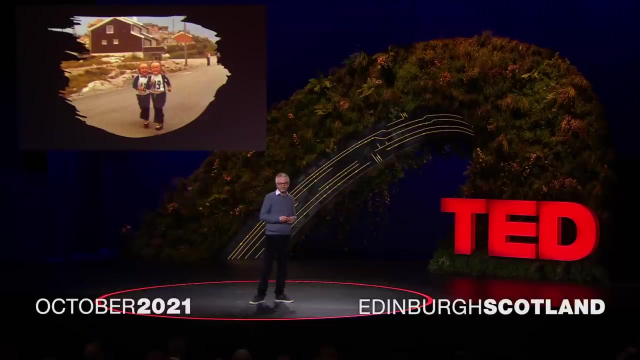 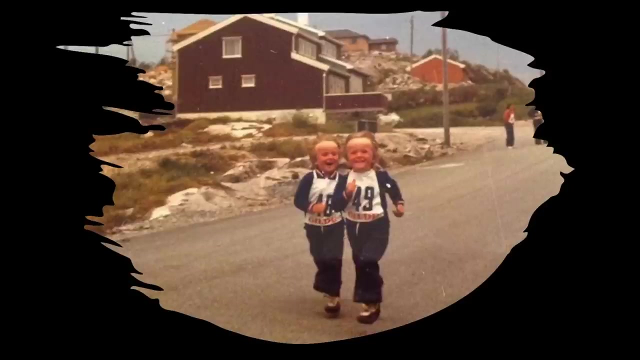 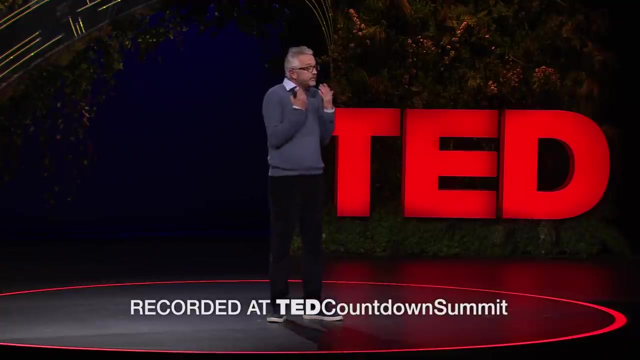 I'm an identical twin. This is a picture of me and my twin brother running a 60 meters race. five years old, I can't tell who's who. My mom can still not tell the difference either. Also, at the time I didn't know that the air we were breathing 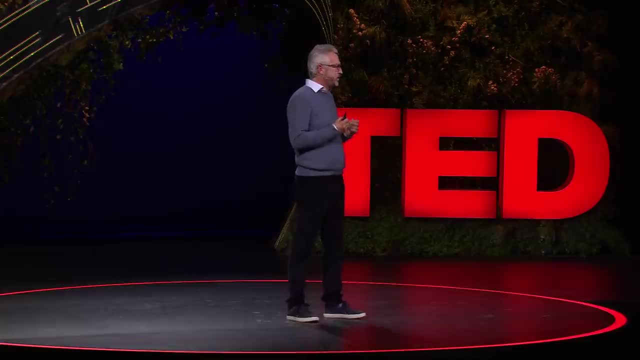 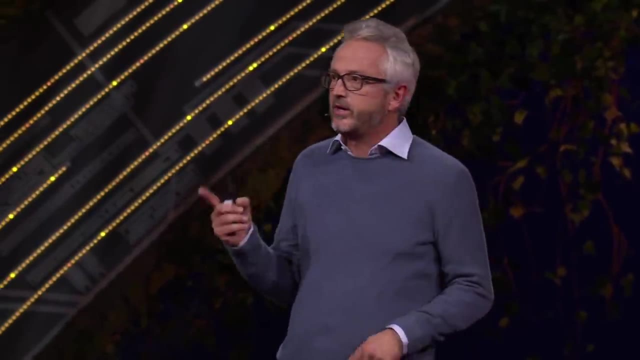 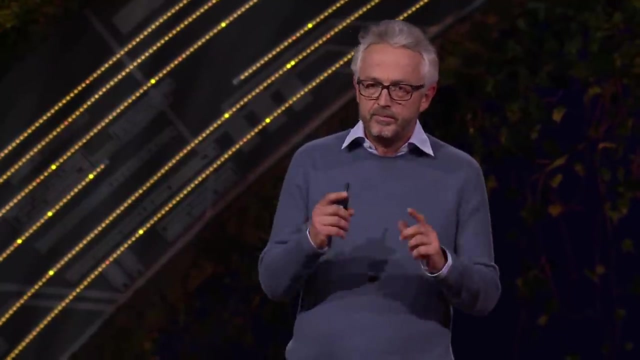 when we were running, had a concentration of 320 particles per million. Today that is 410.. Scaringly close to the 430 threshold. scientists are telling us we need to stay below in order to keep below 1.5 degrees warming. 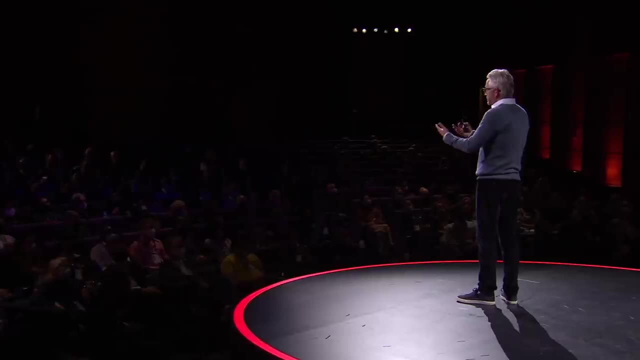 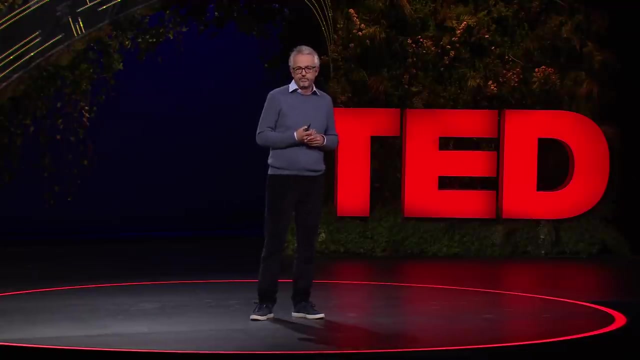 This change has happened in my lifetime, in our lifetimes. A big part of the challenge is the energy system. Actually, two-thirds of the energy system is the energy system. It's coming from fossil fuels. So, basically, we cannot fix climate without fixing the energy system. 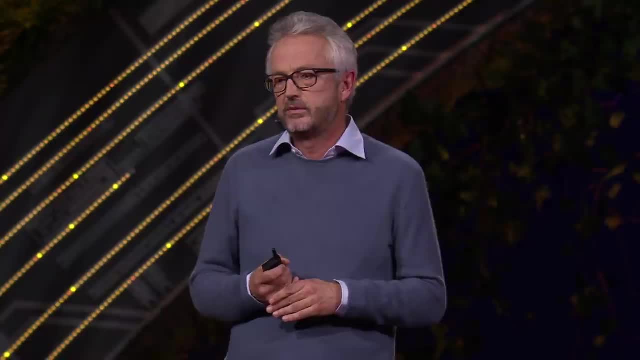 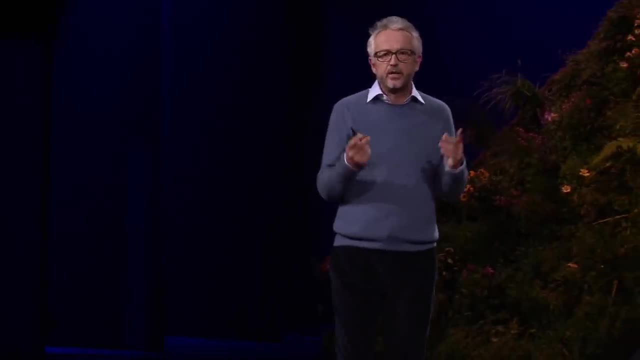 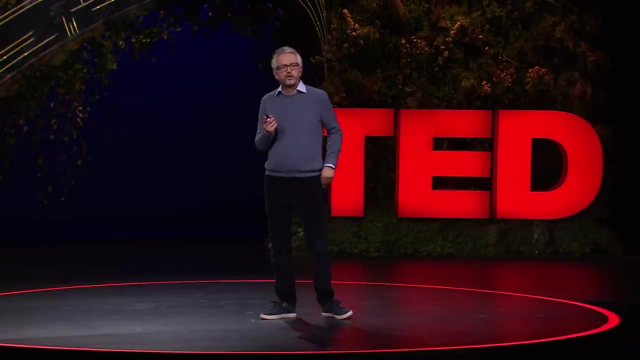 And the one industry that needs to make the biggest change is the oil and gas industry. Many are blaming the oil and gas industry giving up on it ever-changing, being very impatient to see change. I can understand that impatience. I am impatient. 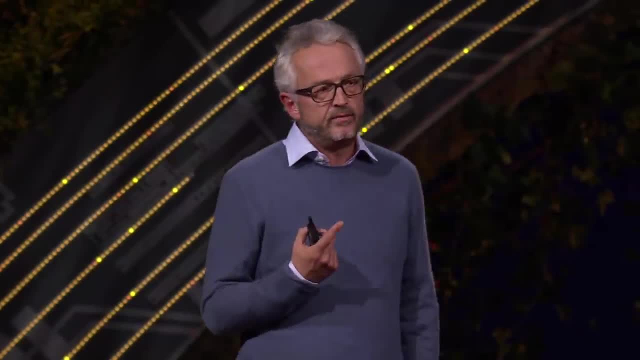 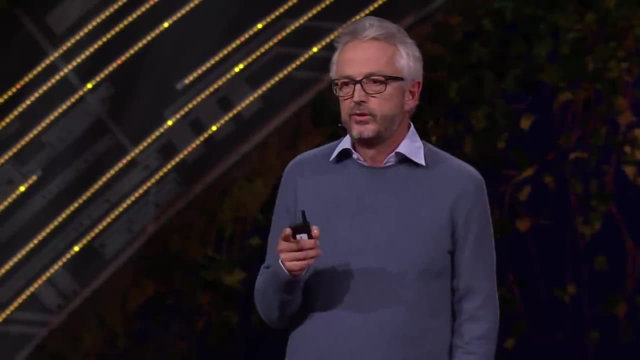 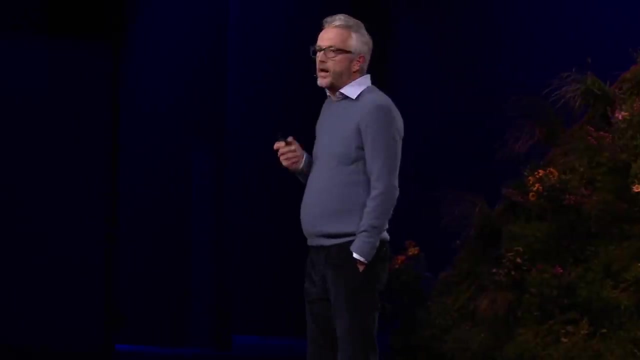 But I still believe that we are better off not ignoring this industry. Let's instead try to turn it into to help drive the change we need to see. Let me tell you why. I lead an organization that's called Oil and Gas Climate Initiative, OGCI. 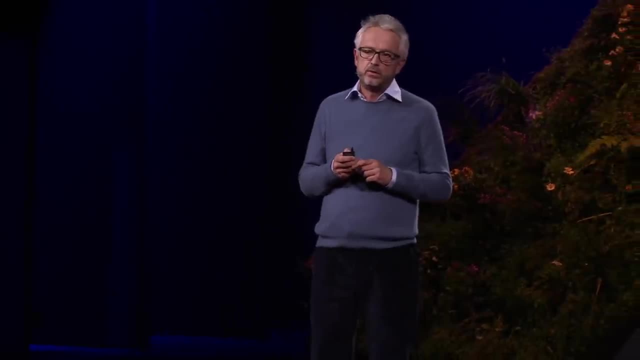 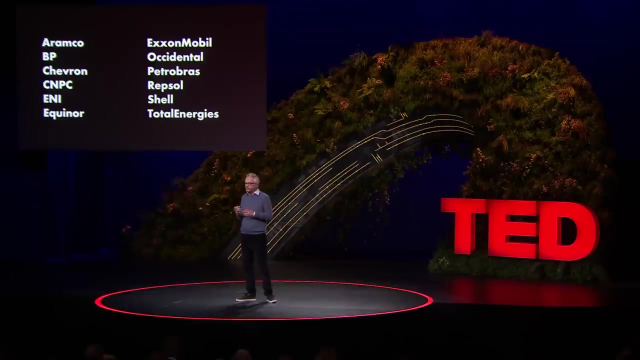 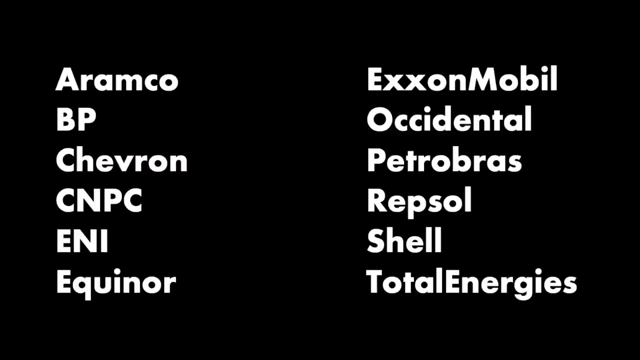 It brings together 12 of the largest companies in the world and their CEOs. The members, as household names, are actually producing every day nearly 30 percent of the world's oil and gas production. Even if some of you would like these companies to just disappear, 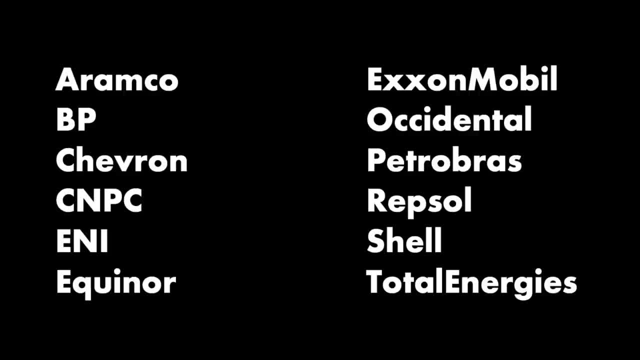 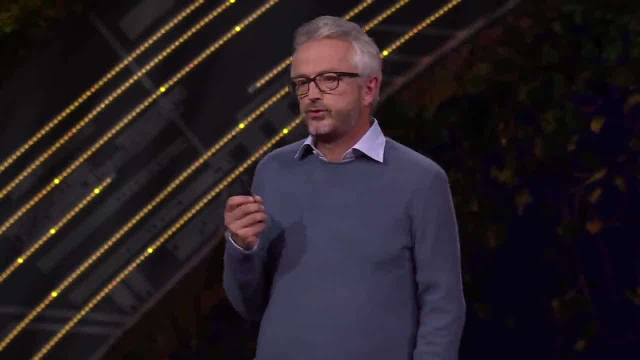 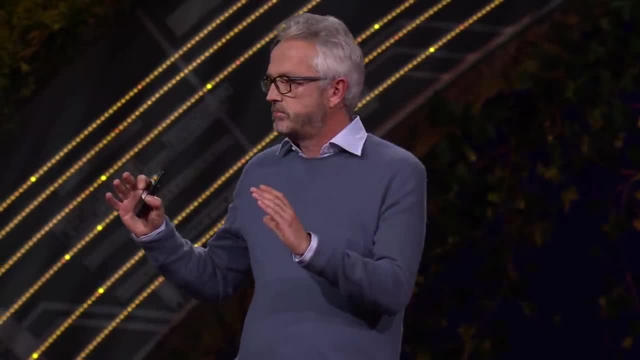 what they are doing matters to all of us every day. Changing the energy system is going to be hard. We need to turn from an 80 percent fossil fuel-based system to a completely sustainable energy system, To a zero-emission system. That would require massive investments. 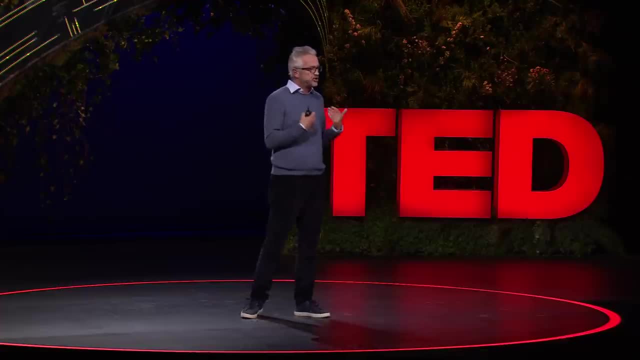 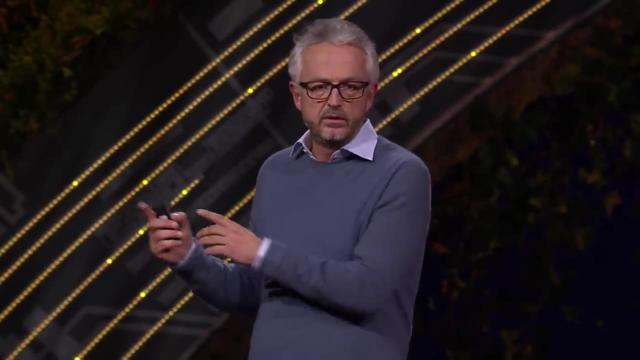 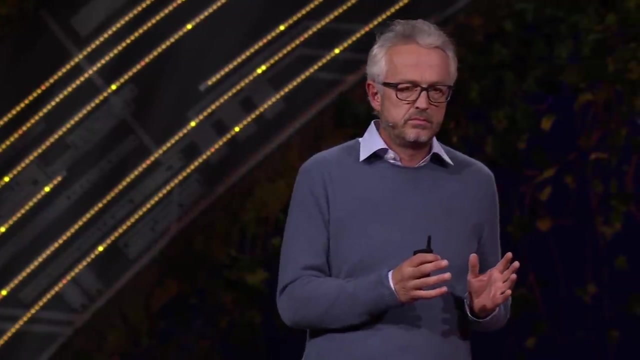 radical policy shifts and us changing behavior. We need to balance that transition with the needs of the nature, fairness, and also to avoid shortage of energy and economic dislocations. And time is very limited So it's very hard to just comprehend the scale of the change. 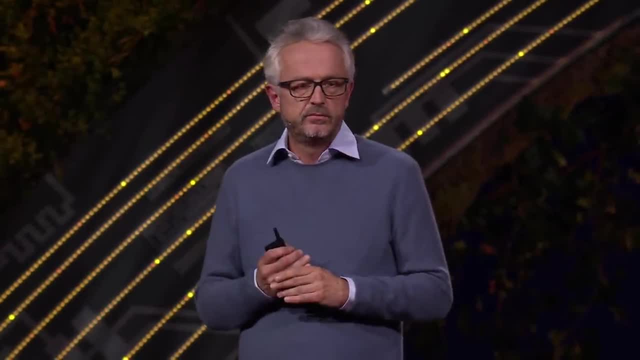 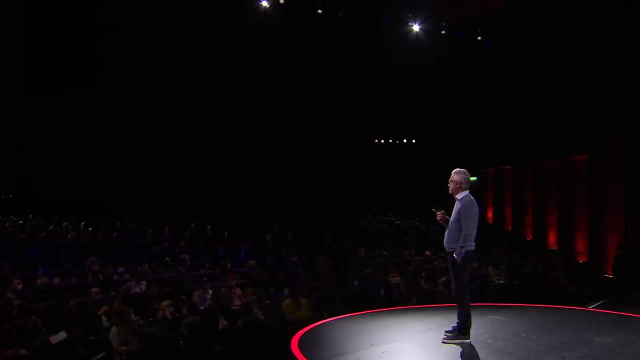 So it's very hard to just comprehend the scale of the change. So it's very hard to just comprehend the scale of the change, But change We must. A handful of companies cannot take on that challenge alone, But we can do more than most. 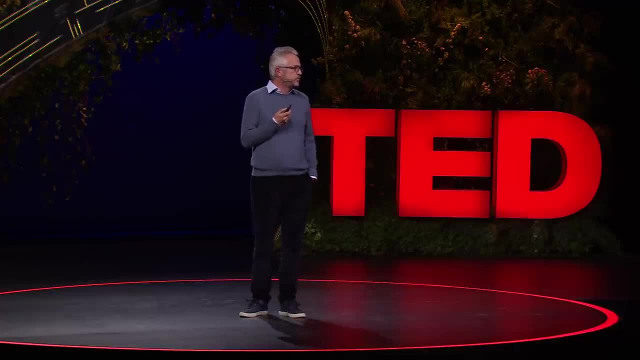 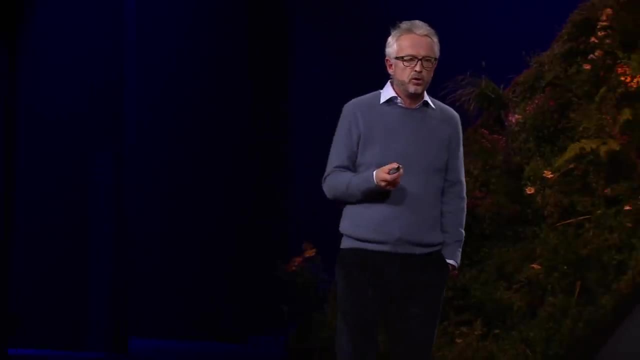 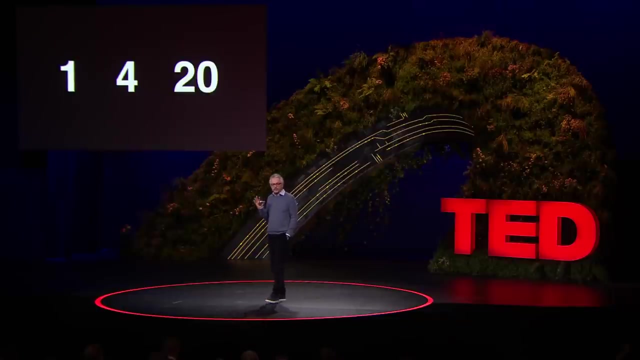 So let me offer you one framework of what I believe we can do and why it matters. I call that the 1-4-20 challenge. That is, one gigaton, four gigatons and 20 gigatons of CO2.. 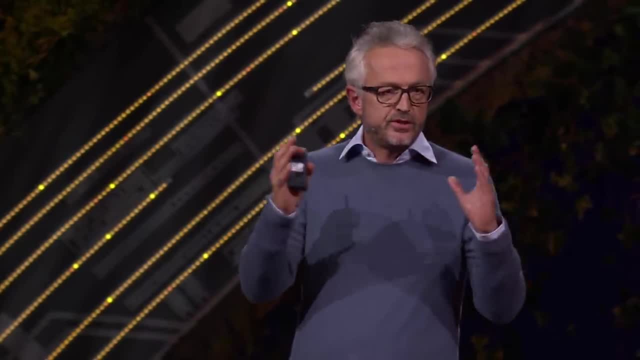 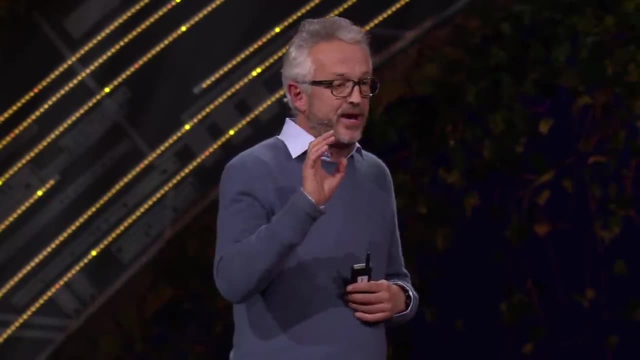 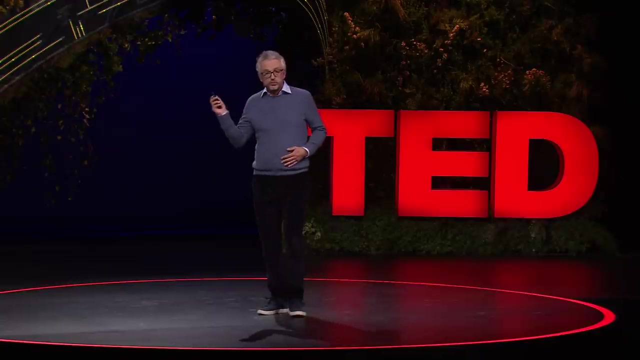 Have in mind, the entire CO2 emission system is 55 gigatons: 33 related to oil, not related to energy, 13 of those coal, And we know what needs to happen to the coal. So the 20 is the sum of the emissions from the oil and gas. 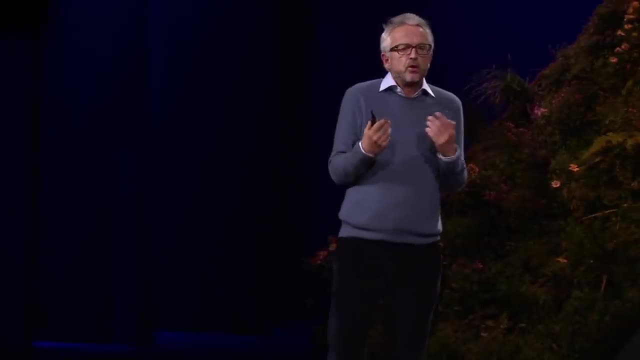 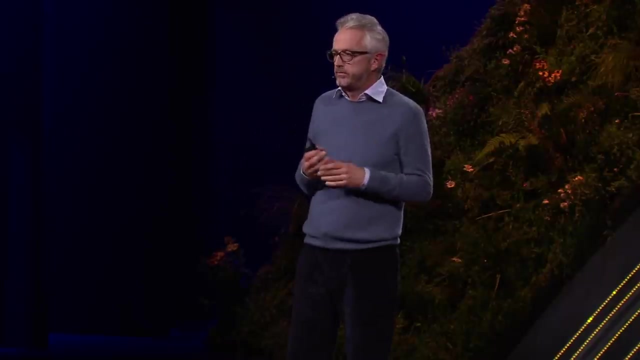 Let's start with the one. So when the oil and gas- the members of the organization is producing oil and gas, they are having emissions, mainly from compressors and turbines, So they use energy to provide energy. right The scope one: emissions. 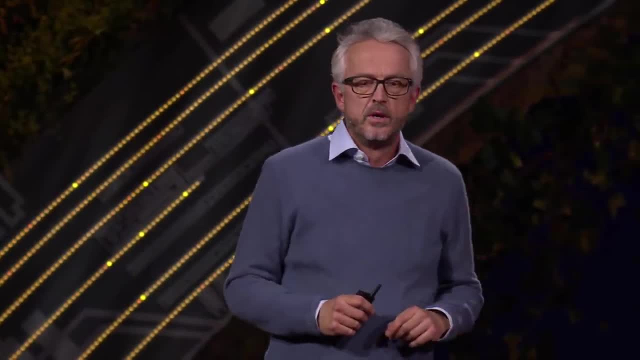 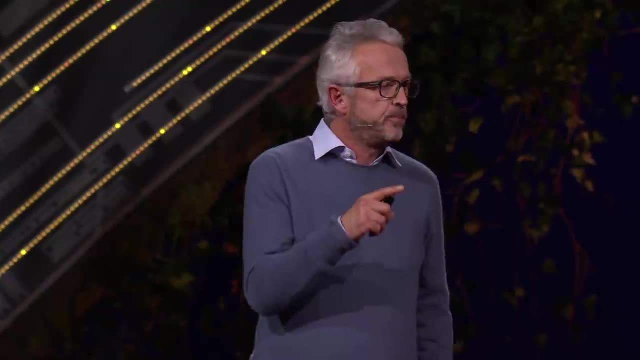 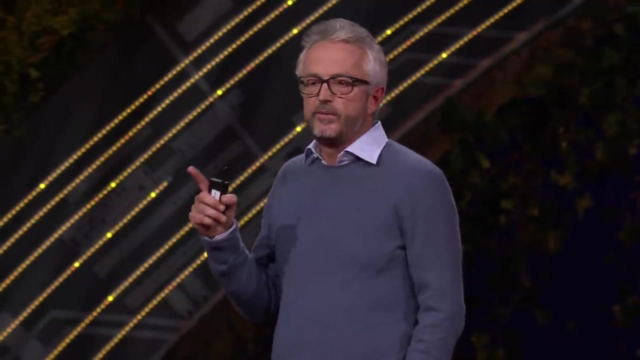 So the first challenge is to bring those emissions to zero. A few weeks ago the CEOs came together and for the first time signed up on the shared ambition to bring all their own emissions to net zero within the timeframe set by the Paris Agreement. 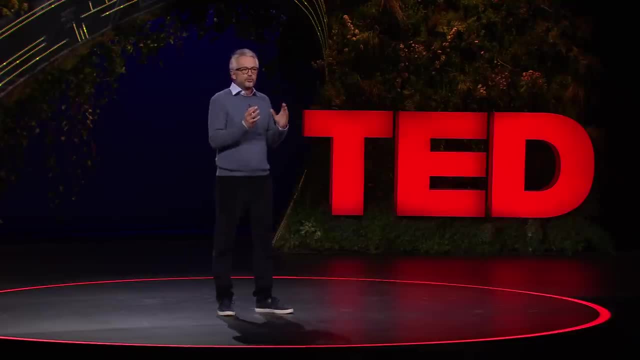 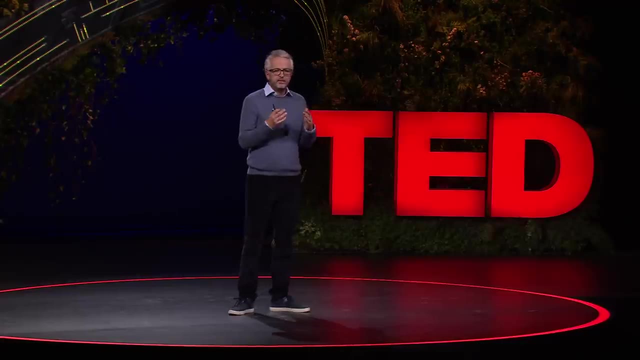 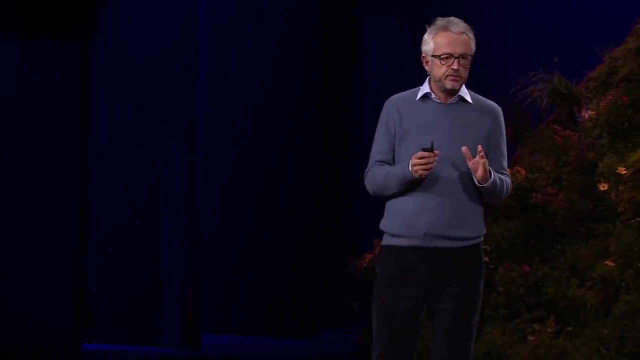 They also promised to leverage their influence to achieve the same in all the fields where they are non-operator. They have never done that before And to me that was a significant step. How are we going to do that? Eliminating methane emissions. 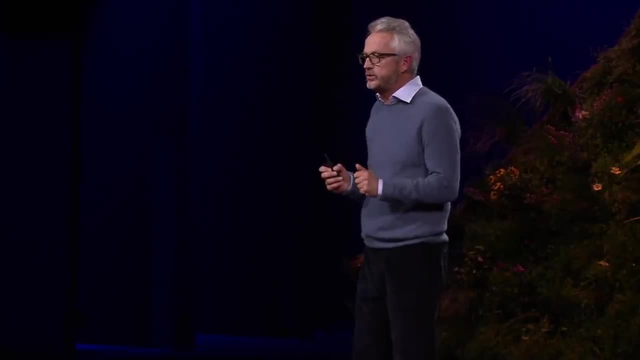 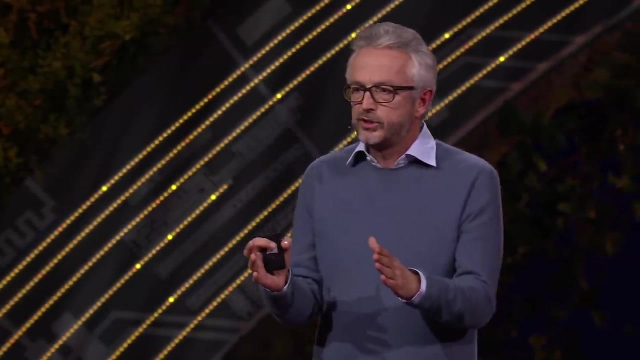 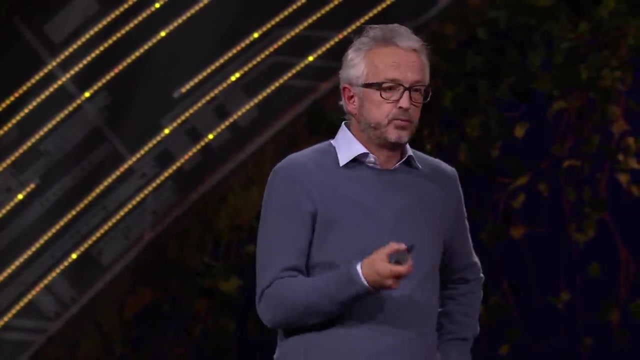 slashing flaring electrifying operations in a bit longer distant future. in a bit longer distant future, we would need to use hydrogen in our own operations: carbon capture and storage and other solutions. Each of the companies would have different ways. 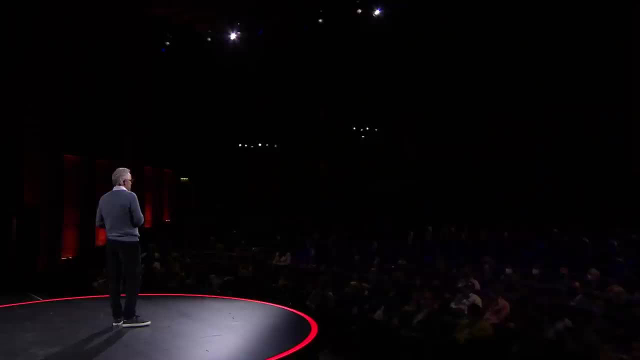 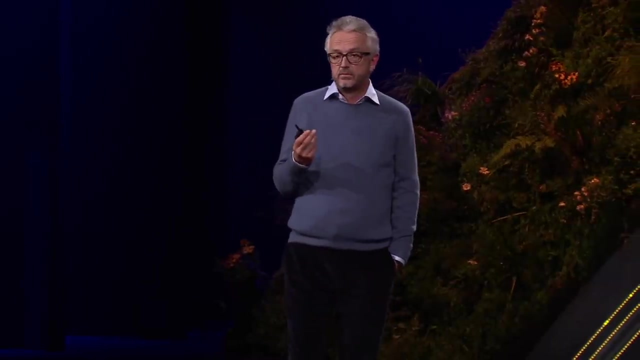 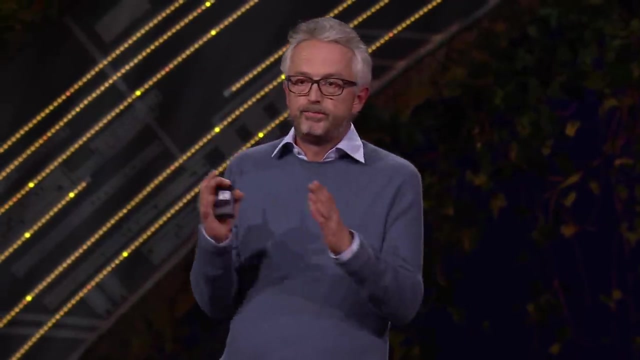 of fulfilling their net zero ambition. You might say it doesn't matter or it's not enough. But daring to say net zero changes minds. It shifts your mindset from one of defensive to proactive, from incremental change to having your eyes on the end goal. 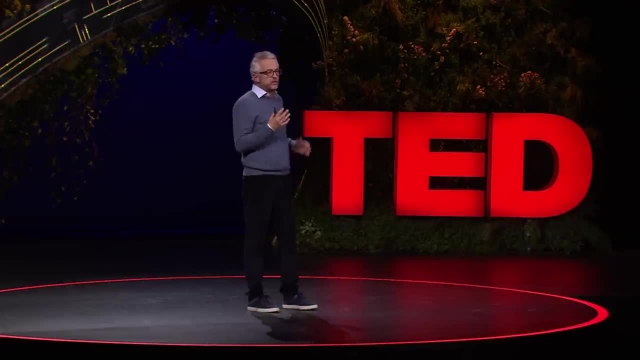 I've seen this happen in my own company called Equinor of Norway. A few years ago, we decided to strive for a net zero. You know what happened: Deep changes in attitudes and behavior of all of the employees started to unfold. 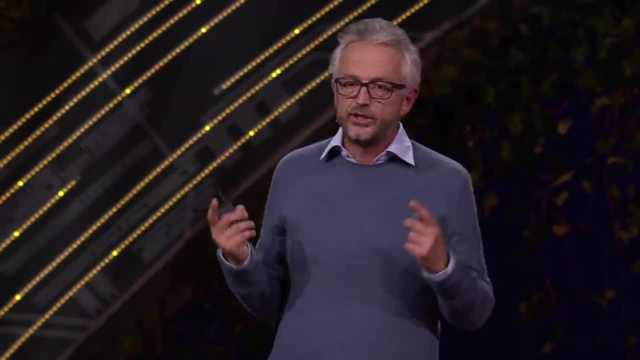 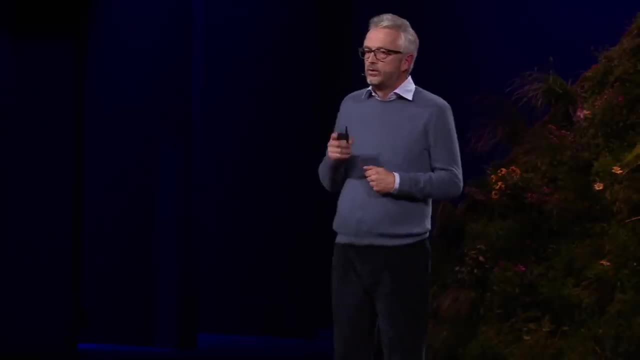 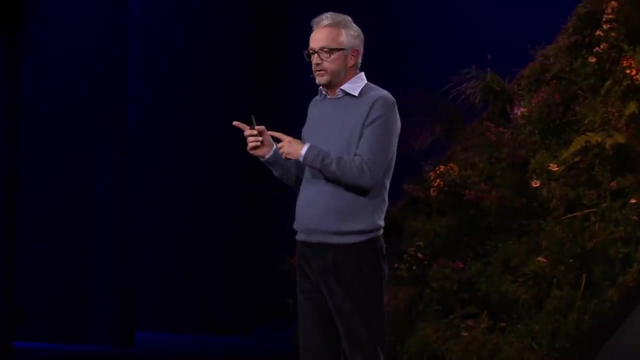 not only among the top management. Thousands of engineers started to look at new solutions. had looked at them differently. Renewables started to become interesting, Investment plans changed. Cash started to flow differently. Now, one gigaton is only a part of the challenge. 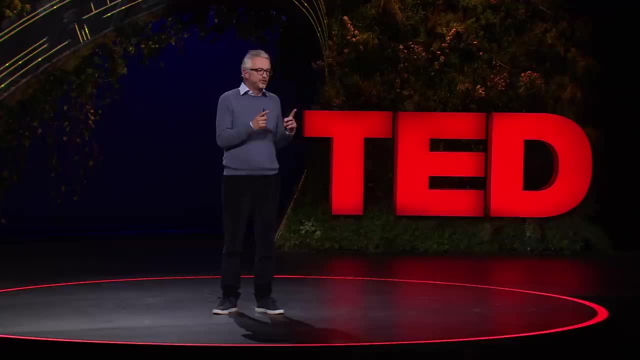 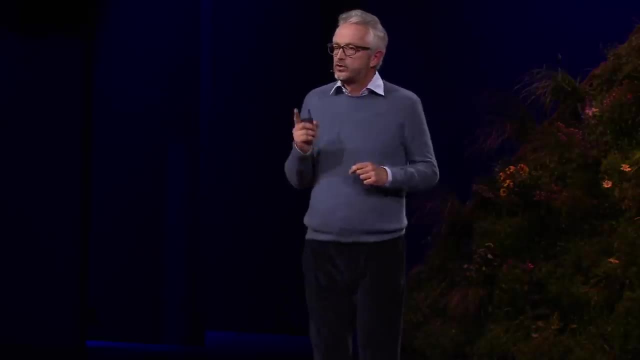 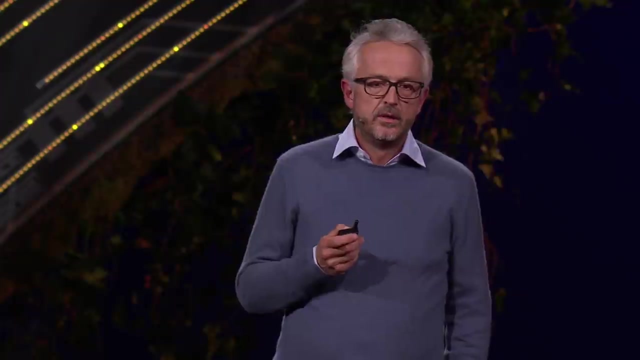 But it's quite big. To put it into perspective, it's the combined emissions of all airplanes in the world, worldwide. So let's try to make that happen. The four gigaton challenge, That is the price if we're able to get all of the oil and gas companies in the world. 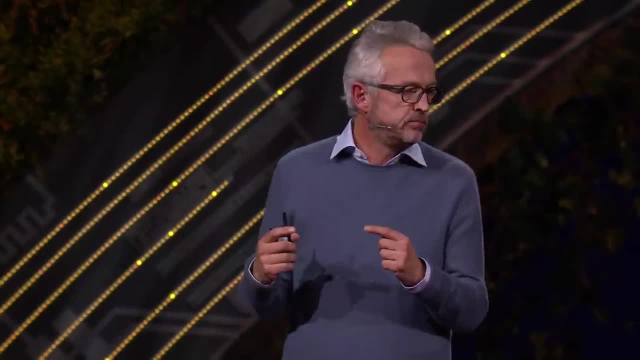 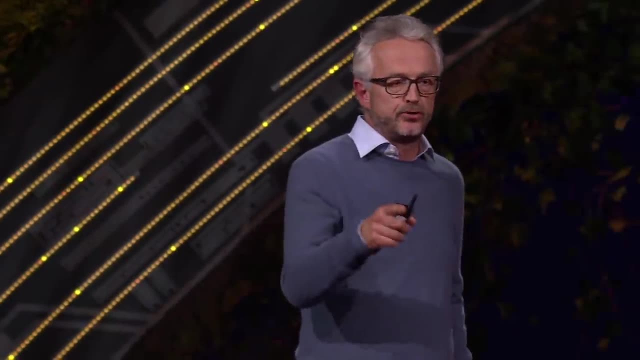 to accept the same ambition: All the national oil companies, all the smaller companies. Four gigaton, I'm going to repeat that number: Four billion tons of CO2 each year. That is equal to seven percent of the world's total emissions. 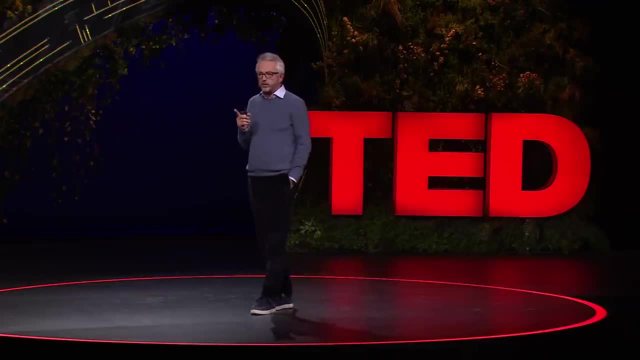 A price that is so big that we cannot ignore it. How can we do that? We believe that we can lead the way by helping to set ambitions, setting targets and also to help countries to identify where it's the problem. We have set targets. 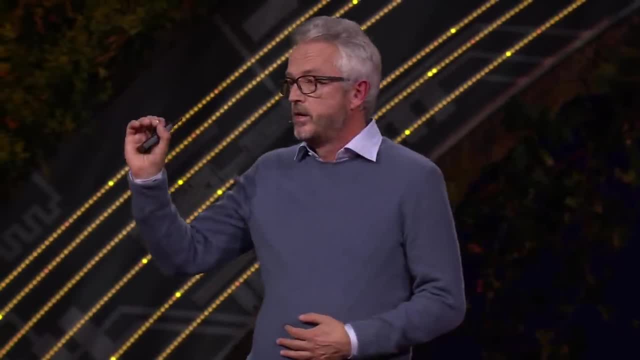 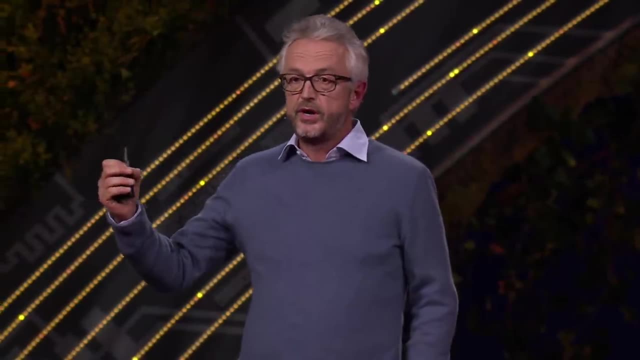 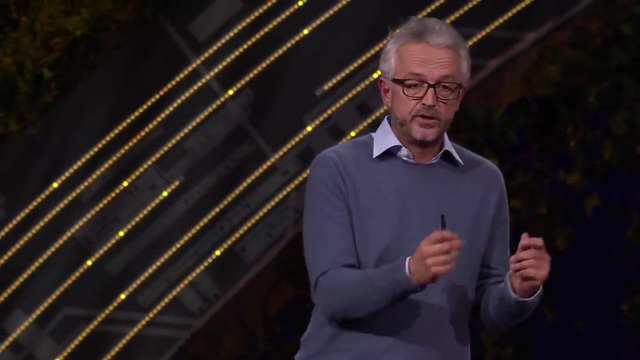 We have also set shorter-term targets towards 2025 for our own performance, But we're also setting targets that can inspire the industry. Recently, we also acquired satellite services To help countries better monitor their methane leaks, for instance- A very big part of the challenge. 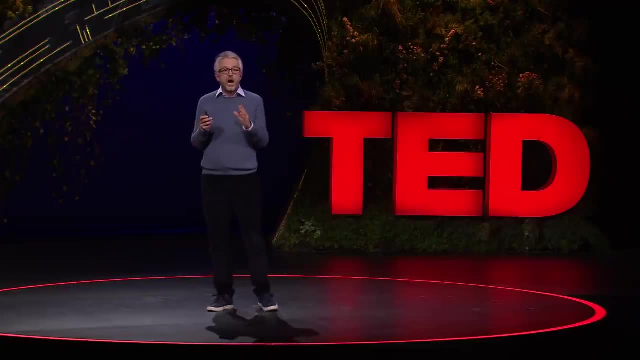 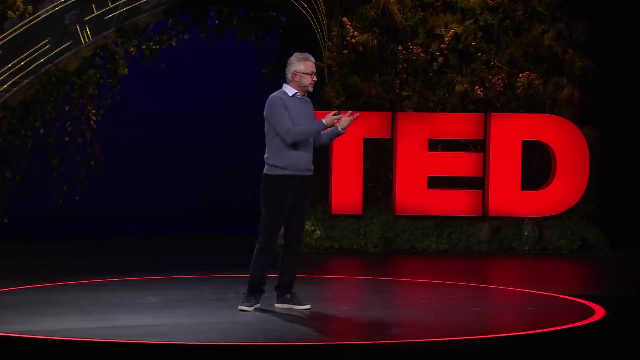 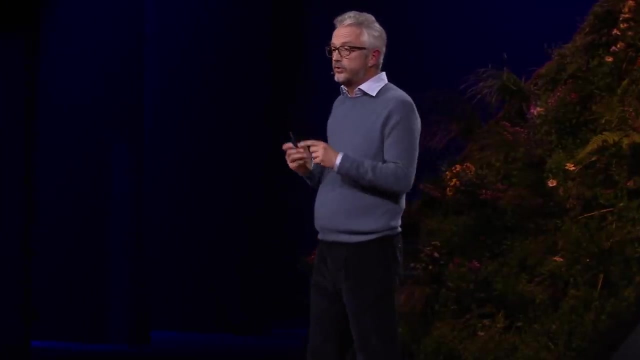 The good thing with this industry: we know how to solve the problems, But we also know that an enabling policy environment will accelerate the change. A particularly important thing is the price on carbon. In some countries $50 per ton will drive change. 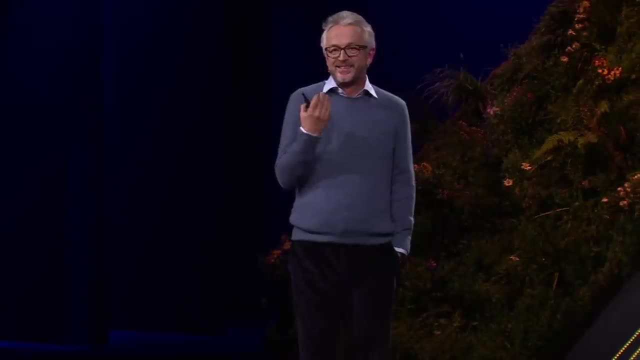 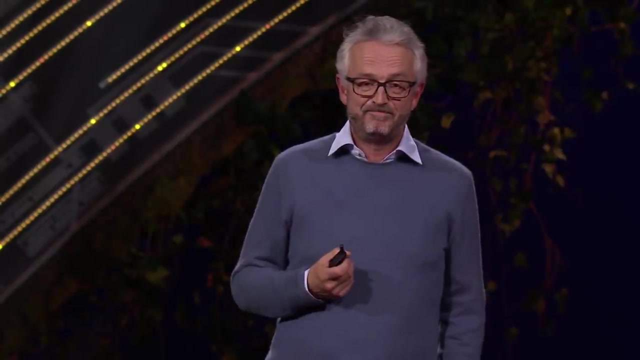 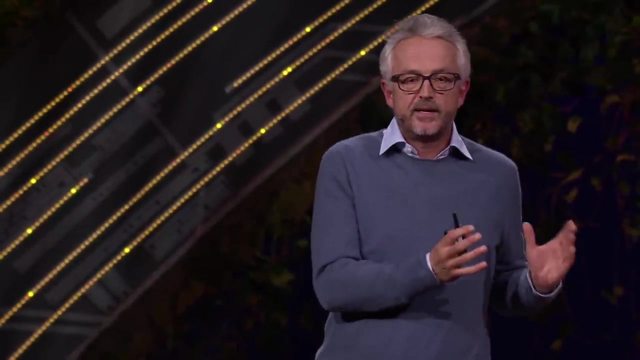 In my own country, Norway, the plan now is to increase that to nearly $200 by 2030.. That is driving change. Now, the one and the four gigaton challenge is both about improving the existing energy system. What we need to do is, of course, 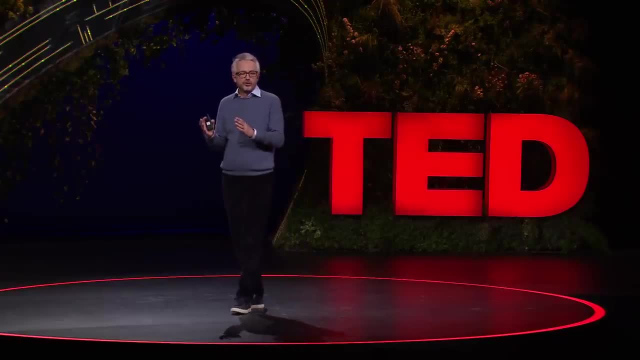 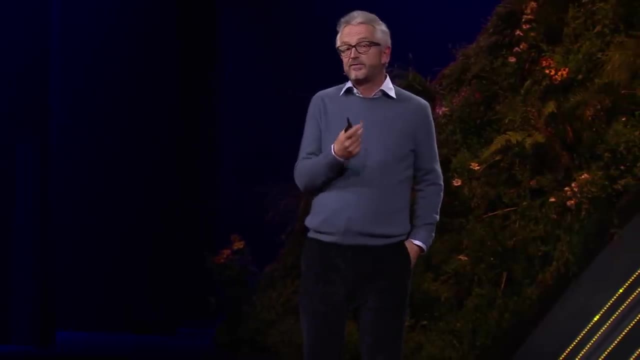 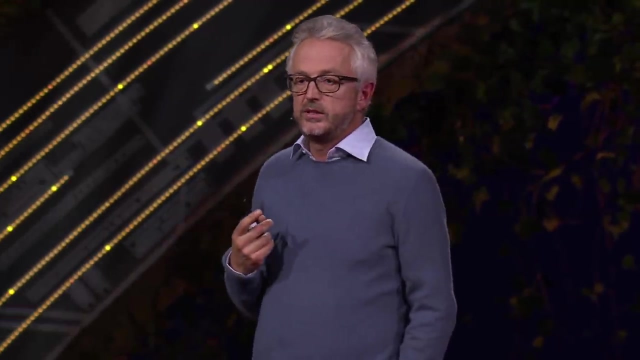 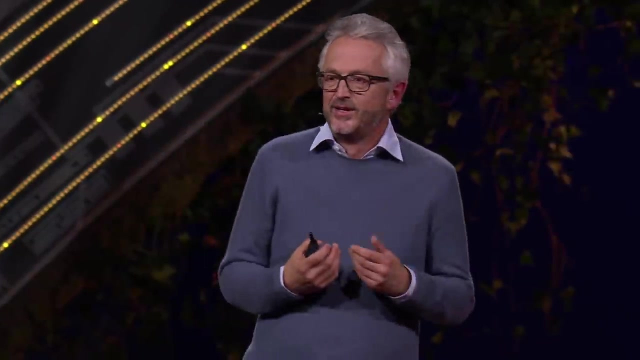 to also build a future energy system, New solutions. The 20 gigaton challenge, as I call it, is a very different challenge. It's a truly collective one. Supply needs to change, as do demand, And we need to find a way of doing that. 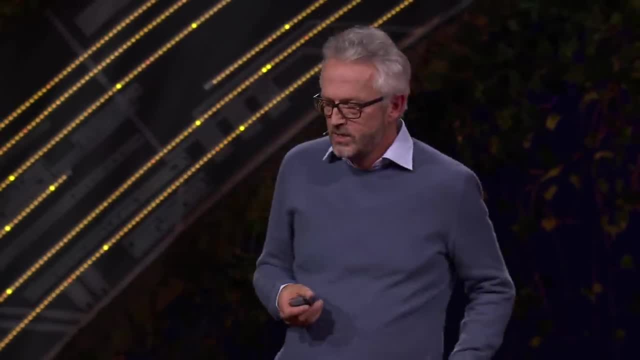 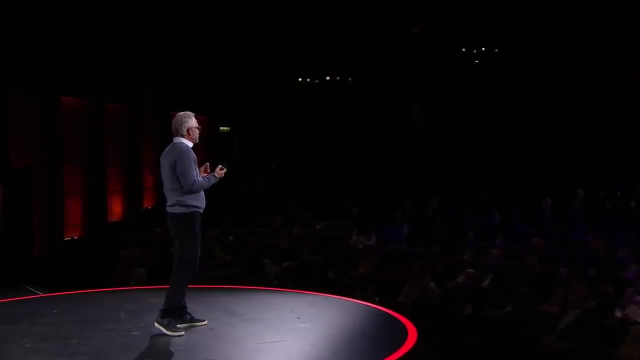 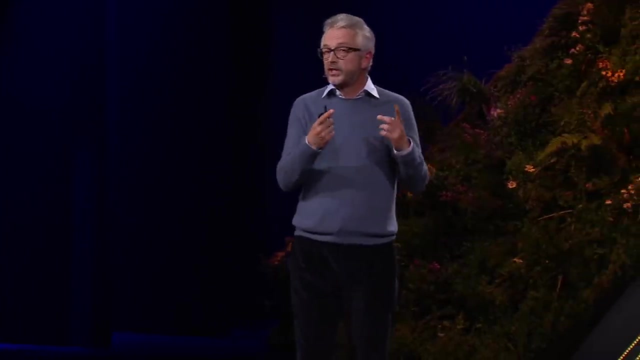 as quickly as possible and as orderly as possible. The oil and gas industry can, of course, decarbonize quicker themselves, but they can also help others achieve their decarbonization efforts. And inside the industry a transformation is underway, Not complete. 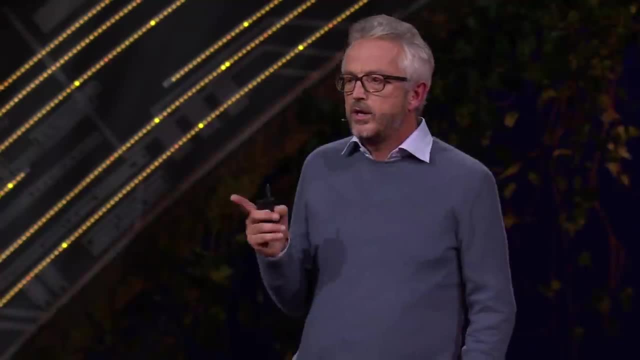 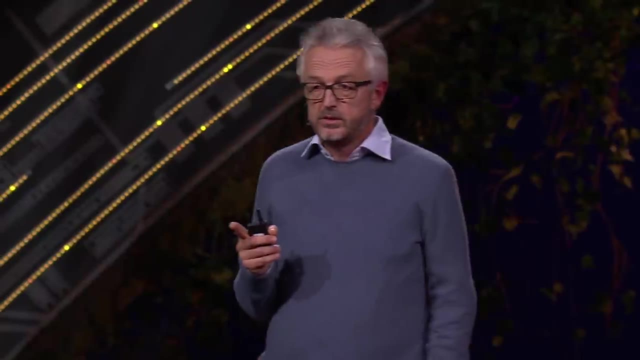 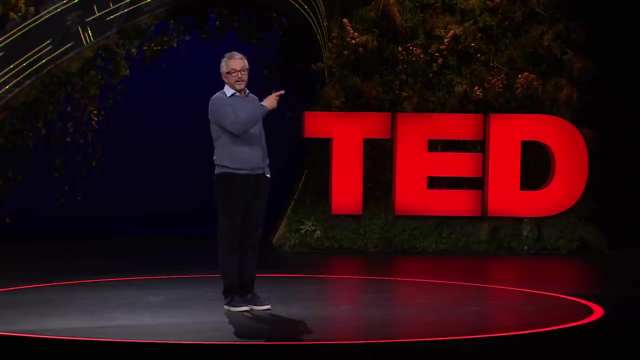 but I dare say underway. Oil and gas companies are starting to see themselves as energy companies and act like it. Renewables is becoming the fastest growth area For Equinor, my company, for instance, the next big, the biggest new project. 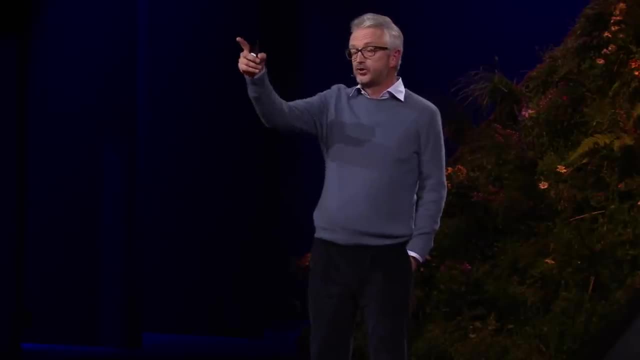 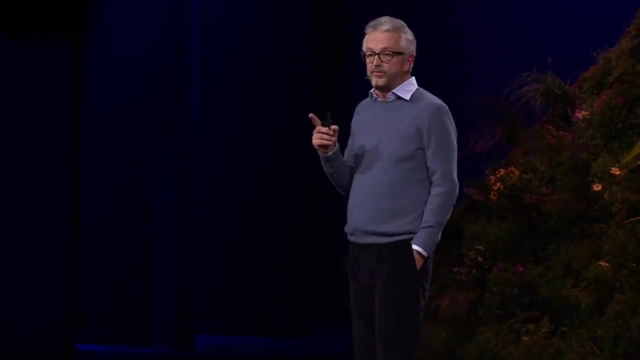 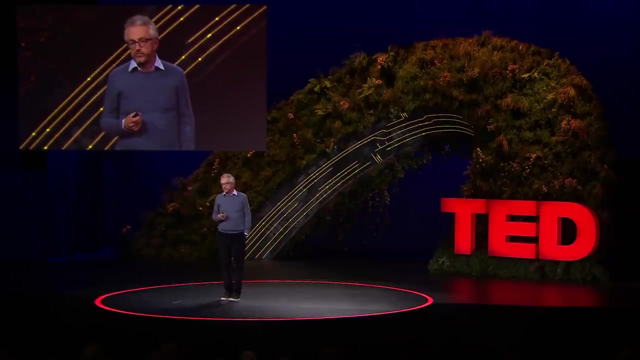 is not another oil and gas platform. It's actually an offshore wind farm development in the North Sea: $10 billion investment with the capability to power 4.5 million homes in the UK. Further up north in the UK, Shell, BP and other companies. 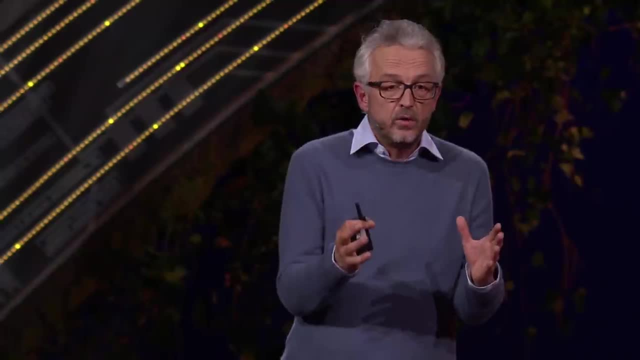 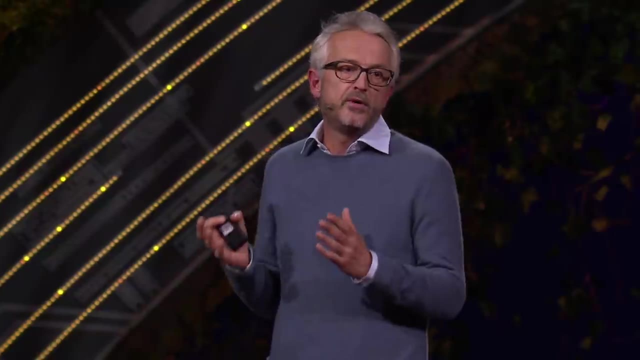 are involved in developing carbon capture and storage industry. That will help cement steel and other industries meet their climate efforts. This used to be future music, but now it is happening. Seven of those projects are underway. We believe they can be materialized by 2025. 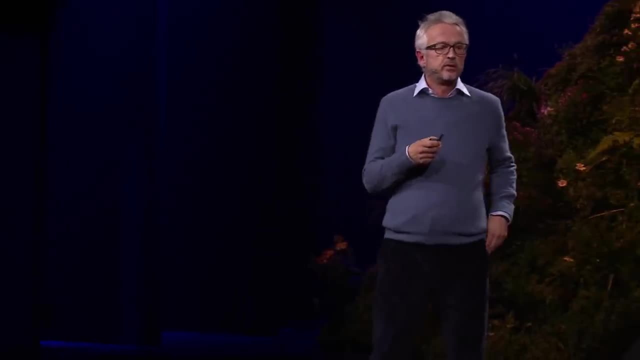 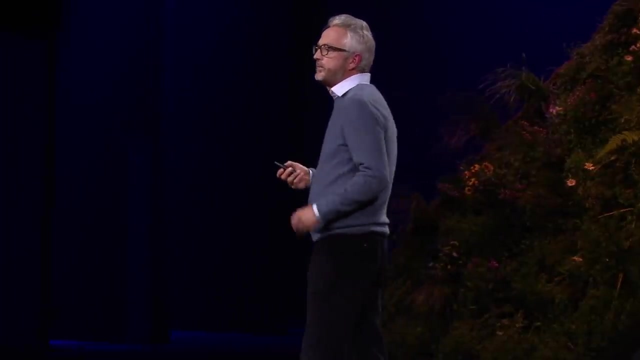 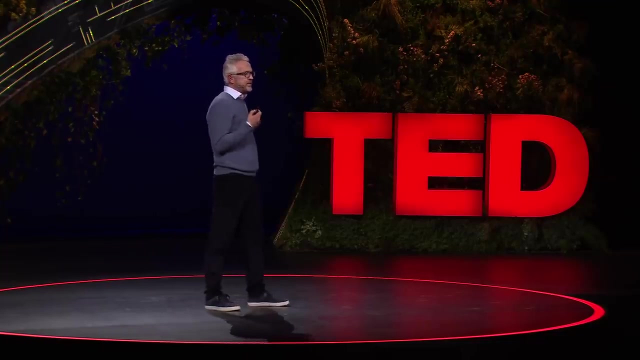 More than 25 other projects are ongoing. Similarly, in hydrogen synthetic fuels, biofuels. quite a lot of things are happening For me to unlock the potential, the scale, the capacity, the competence of this industry to put it to work. 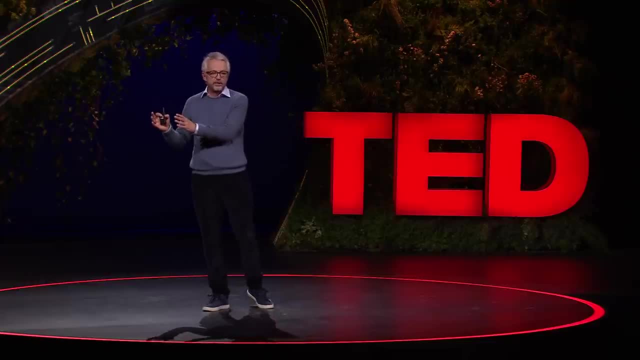 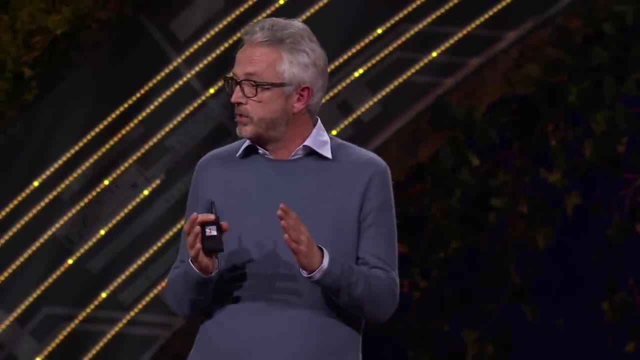 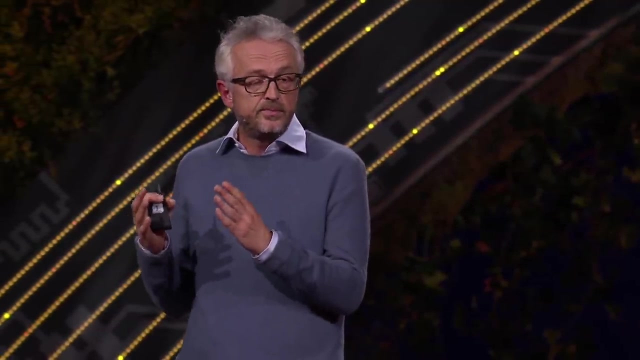 to drive the broad transformation of society that we really need is what motivates me Not to speed it up, not to slow it down. Then we need to act and use our voice in accordance with the spirit and the consistency of the Paris Agreement. 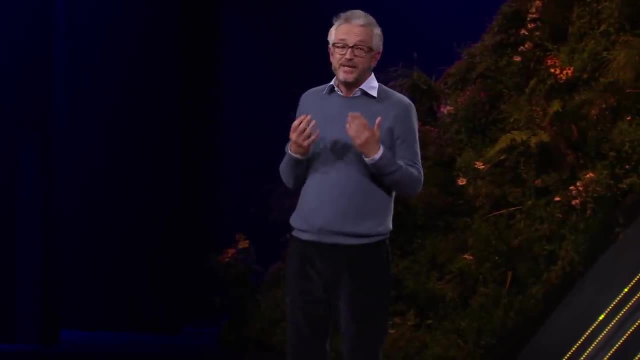 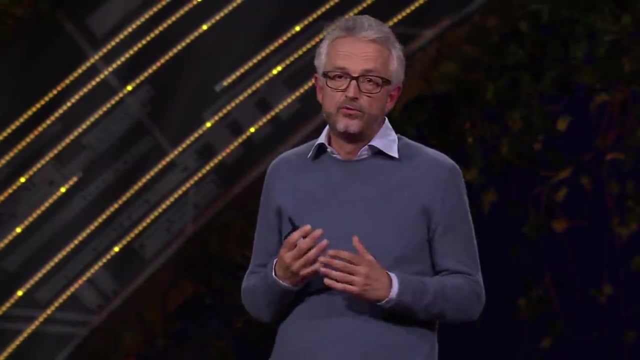 This is what inspires me And I know, of course believing is important, but at the end of the day, we will be judged by how we are actually delivering on the 1,, 4 and 20 gigaton challenge. The race is on. 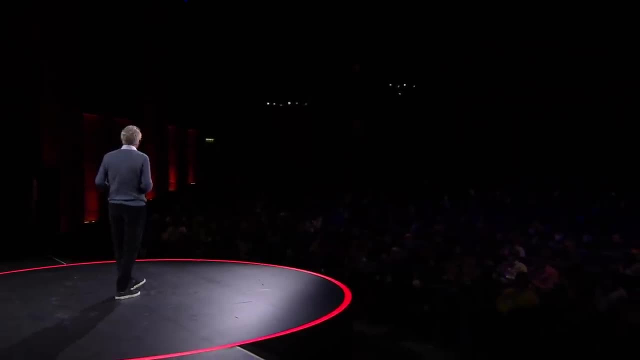 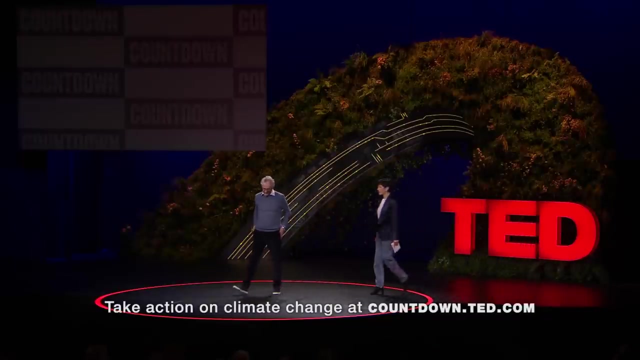 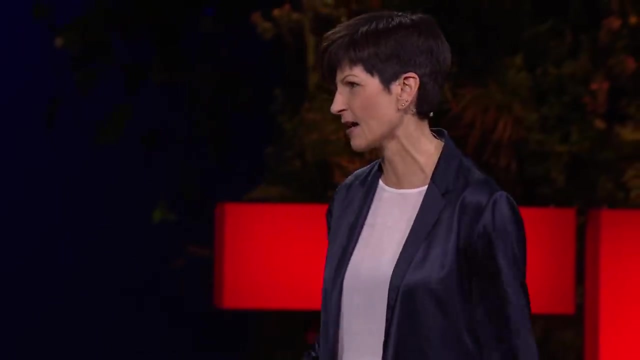 Thanks, Bjorn-Odo, thank you, Thank you very much for that. Thank you very much for that And help us square the circle here, because, in the meantime, so many of these companies continue, continue to push for new exploration. 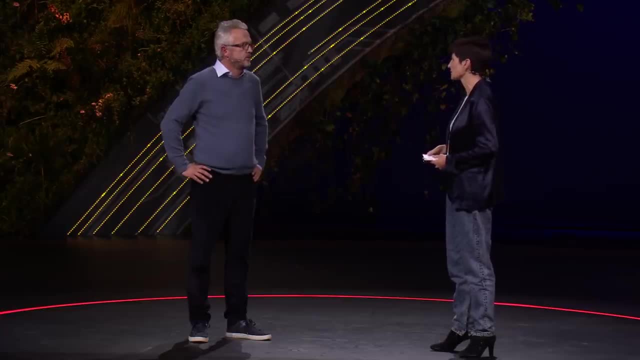 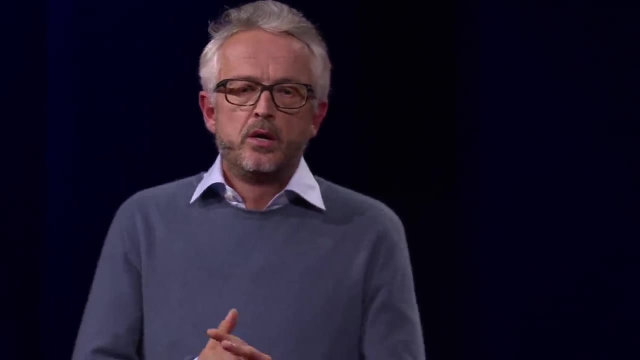 How do we make sense of that with the story that you've just shared? This is a very important question. So, should you continue to explore? Should you continue to produce? What should you do with that? And I think, if you just look at the numbers, actually, the world's total exploration for new oil and gas has dropped nearly 55 percent over the last years. It's at the lowest level in 16 years. So I think things are changing. Some companies are already guiding that they'll plan to reduce production. 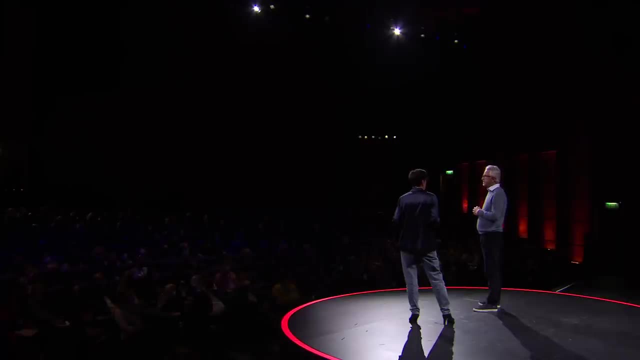 I think all of the companies are recognizing that if we're going to meet the missions of the Paris Agreement or just, you know, have a habitable climate, oil needs to decline, right? So the question of timing. So how do you balance that? Do you? You cannot really stop delivering a product that society isn't ready to not use anymore. So I think if we would really like to accelerate a decline in production of oil and gas, shift the demand right. So make sure that we have seen lasting changes. 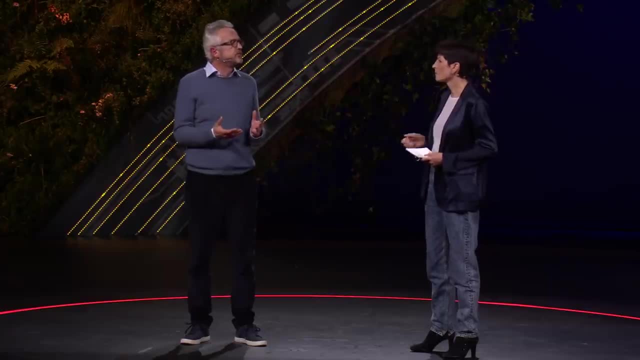 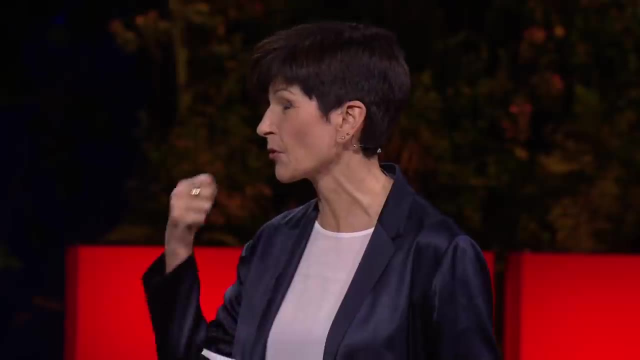 in much more use of electric cars, much more investments in renewables, etc. And at the same time, of course, these same companies are lobbying against a lot of that change. So you know, known for disinformation and misinformation. Could you just speak to us a little bit?